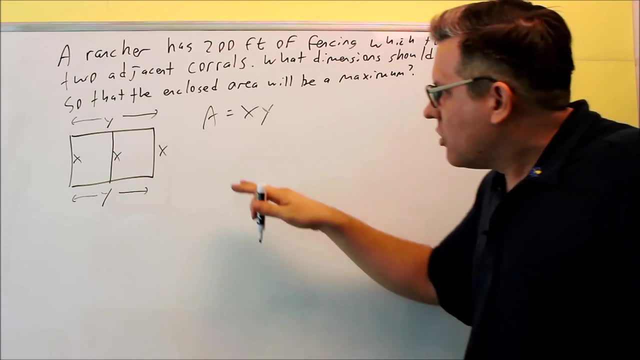 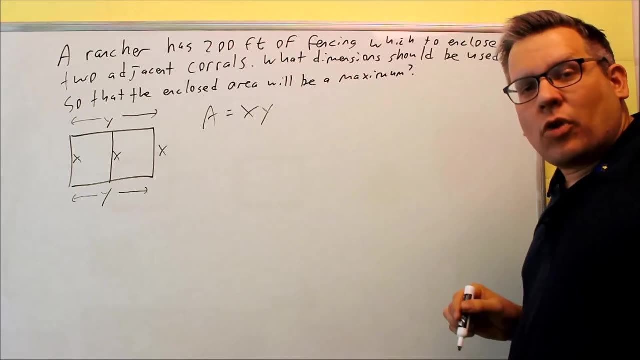 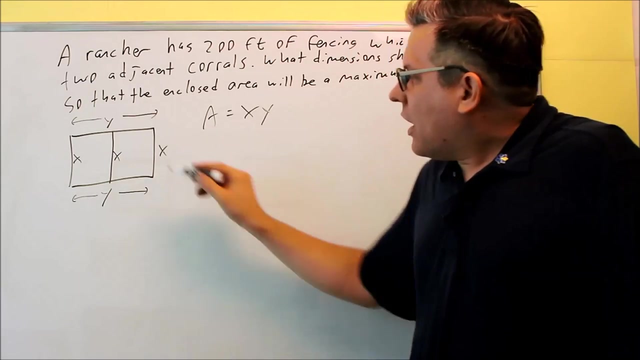 derivative with this because it's too many variables. I want to first find another equation that I can use to substitute back in. We've got to use this 200 feet somewhere. 200 feet is used to create all the different sides of this corral here. So I have three x's and I have two y's. All of that is going to be. 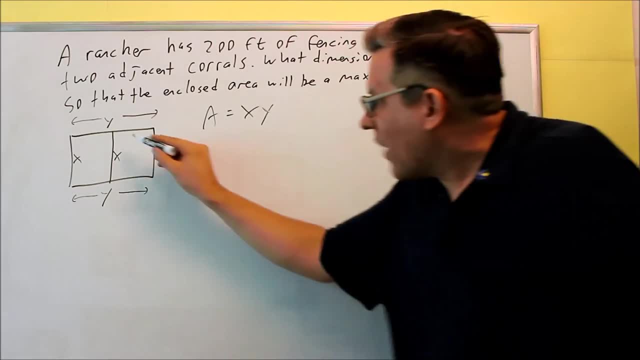 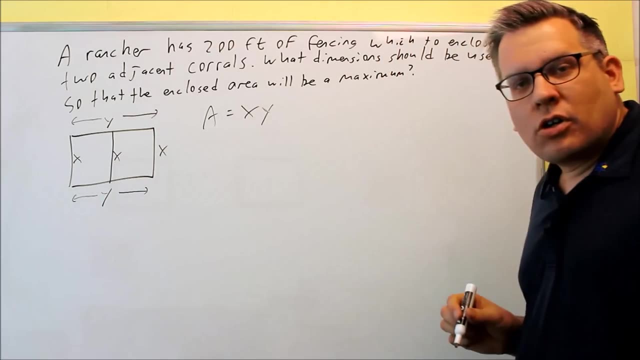 using part of the 200 feet for the material, So we have to include the one in the middle also, because there's material that's being used to make this into two sides, So that's going to make this into two separate corrals. So let's write the equation for this. We. 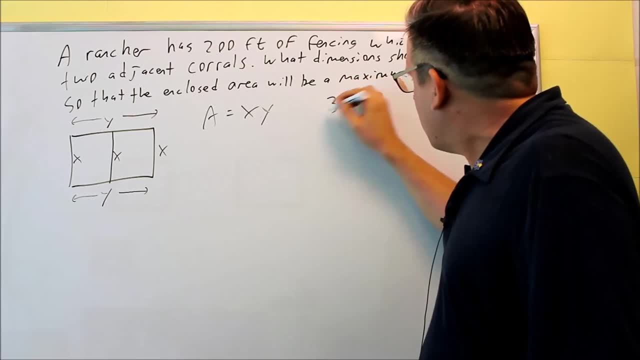 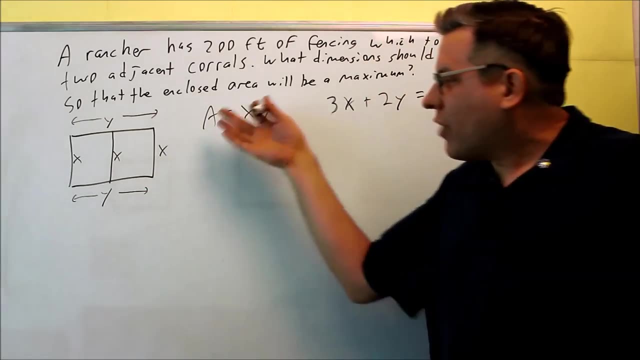 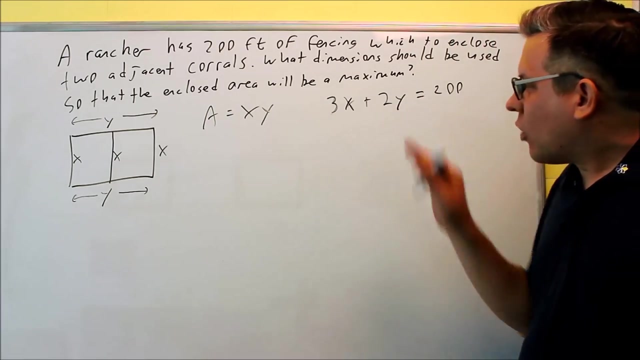 have three x's plus two y's. That's going to give you 200 feet. We have five different pieces to this, and they're all going to add up to 200.. Now what you can do here is you can solve for either x or y, It doesn't matter. Put it into here and then we'll take the. 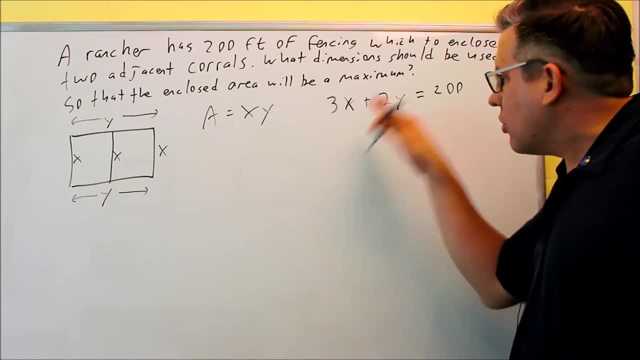 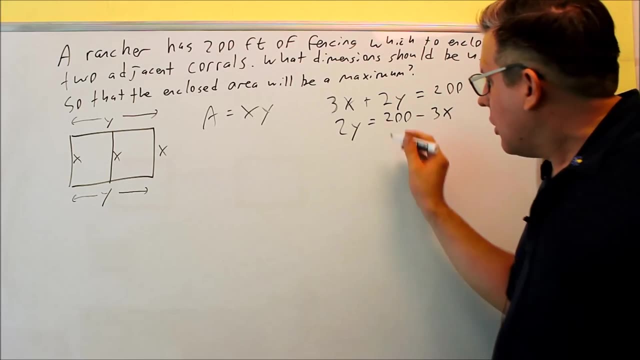 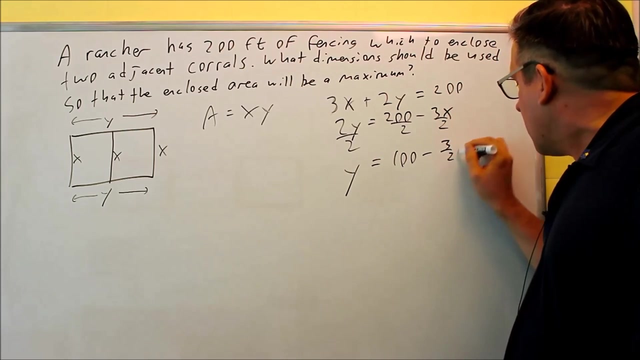 derivative. I'm going to solve for y in this case, but again, you could do either one, It doesn't matter. So y is going to equal 200 minus three x and I'm going to divide everything by two. So I'll just do each of these separately. Y is equal to 100 minus three halves x. I'm 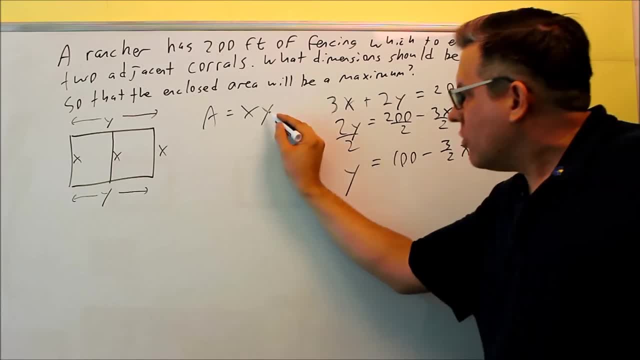 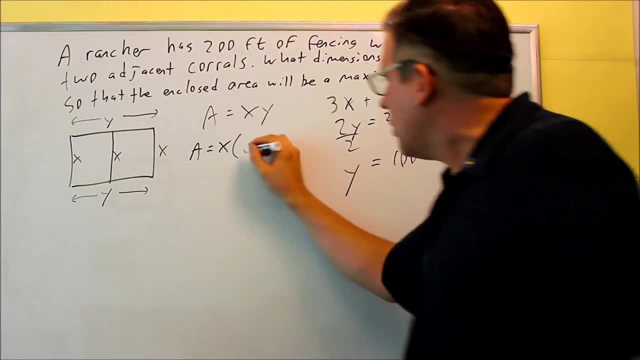 going to take this y, I'm going to substitute it back into that y right there and I'm going to get x times instead of the y. I'm going to put in this right here: 100 minus three halves x. Okay, 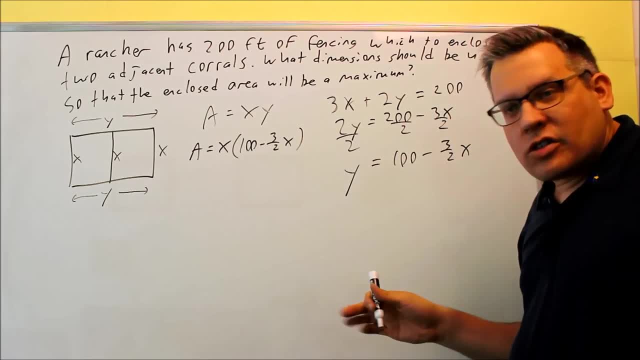 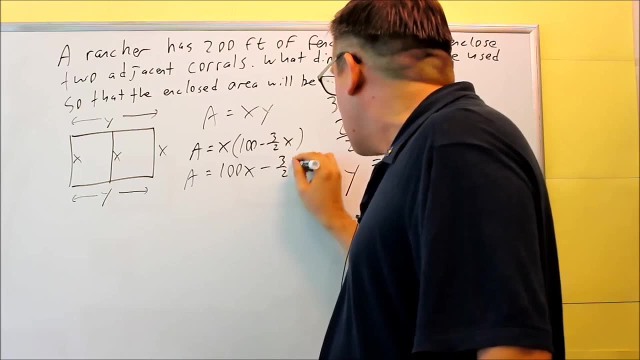 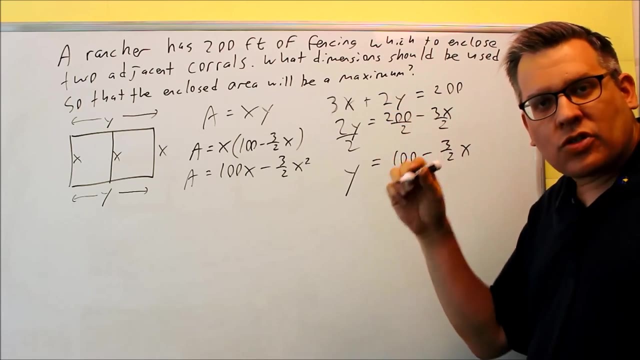 So this is your area formula. Now, if this was a precalculus class, I would multiply this out, which I'm still going to do anyway here: 100 x minus three halves x squared, and I would apply negative b over two a to find the vertex, and the vertex corresponds to the. 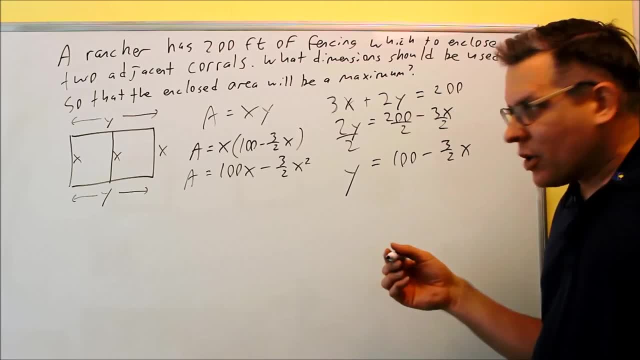 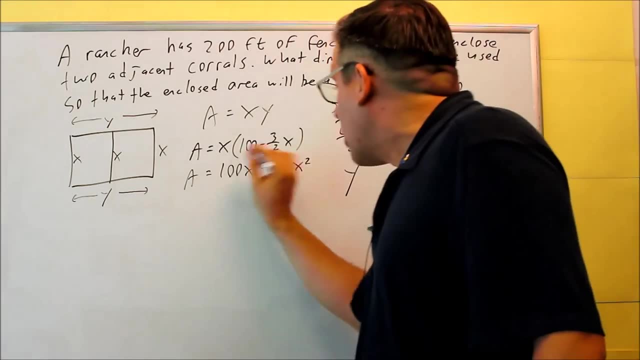 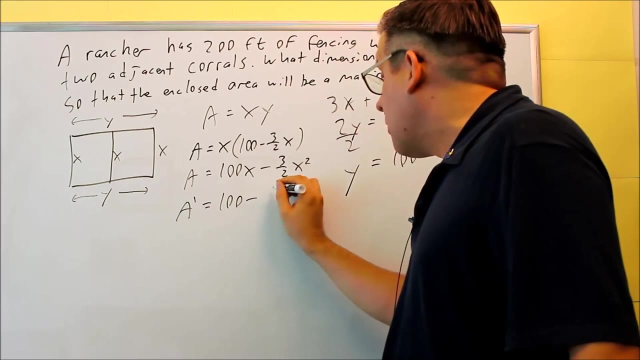 highest or lowest, because we have a quadratic here. However, because this is calculus, instead I'm going to take the derivative, set it equal to zero. So here's our original function. I multiply it out So I could use the power rule: Derivative of 100. x is 100.. This is a primed here Minus.